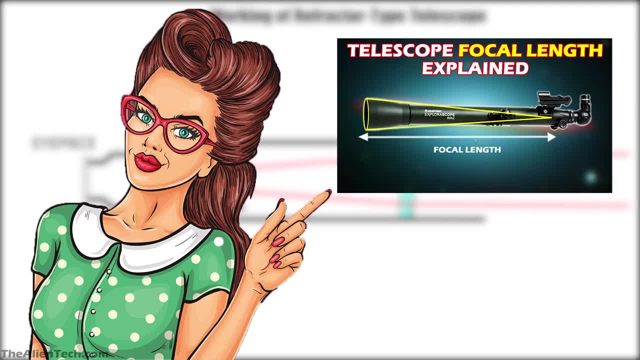 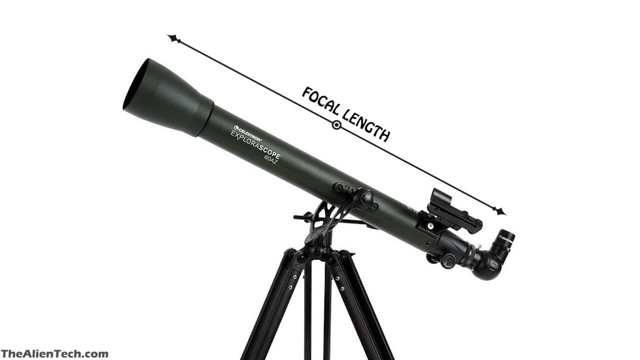 If you want to learn more about focal length, then you should watch this video. If the focal length of a telescope is longer, then you can get maximum magnification with that telescope. When telescopes were invented, at that time, every single telescope was a refractor. 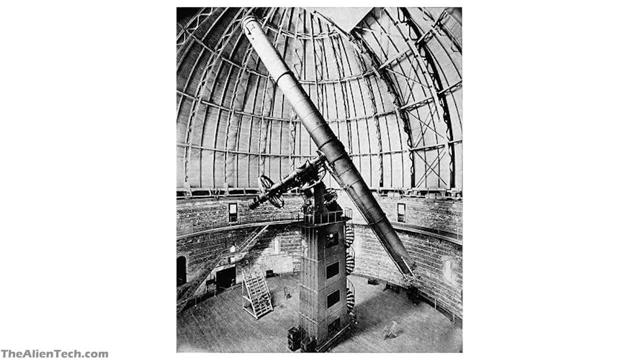 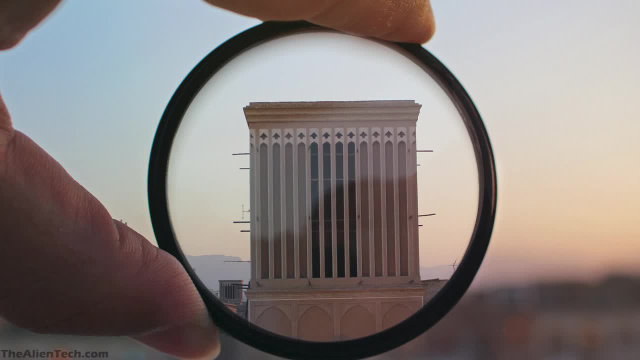 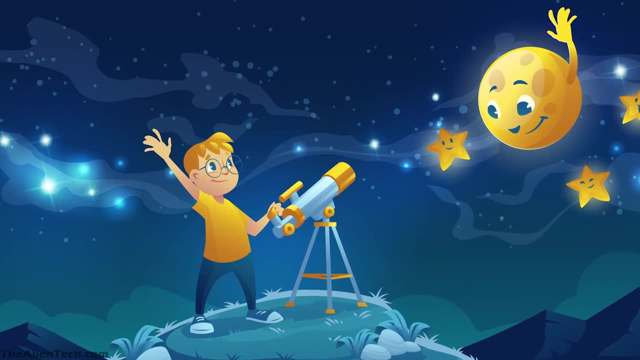 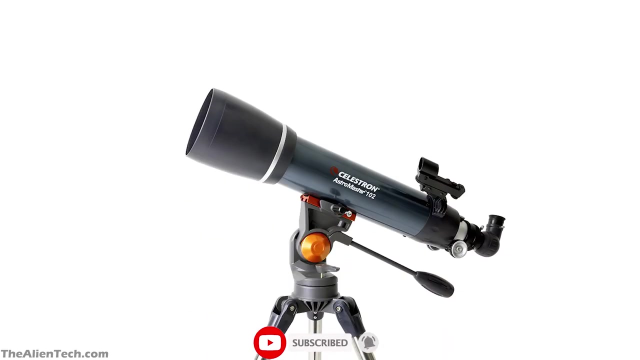 telescope. So to get more magnification they built very long tube telescopes. The refractor telescope uses a lens instead of mirrors. Refractor telescopes get very expensive as the aperture size of the telescope increases. Manufacturing a big aperture refractor will need a big lens. So most of the refractor telescopes 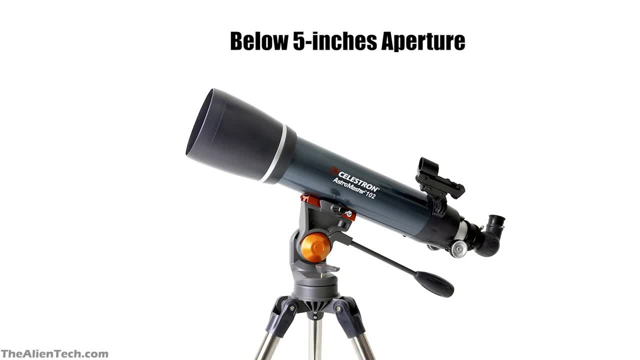 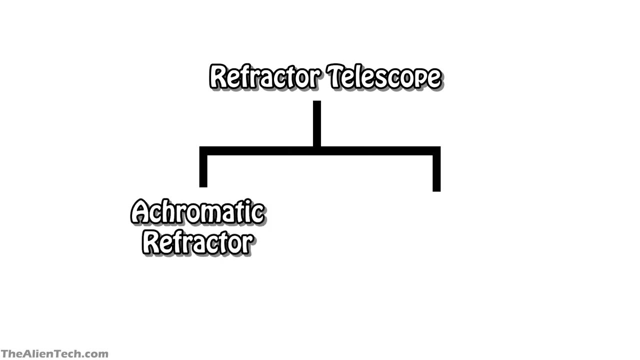 you will find, have an aperture below 5 inches. The refractor telescope is further divided into two types – an achromatic refractor and an apoachromatic refractor. WHAT IS THE DIFFERENCE BETWEEN THESE TWO TYPES? 2. Maples are very similar to lavalieria's. The signal frequency of the radioactivity of a ray of light is 2- grabs and follows the light about each degree of view. Parallel- Chemistry of the refracting taking". 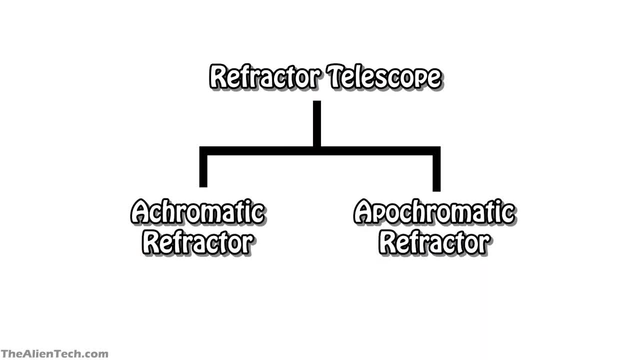 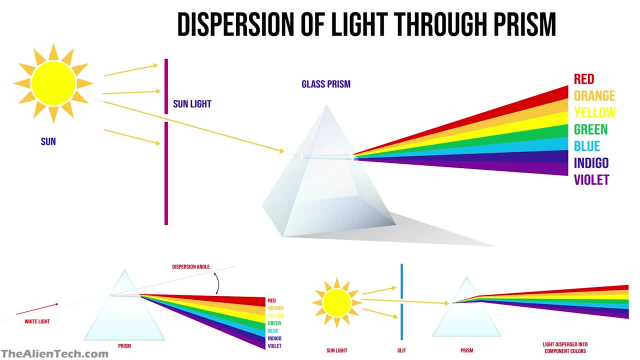 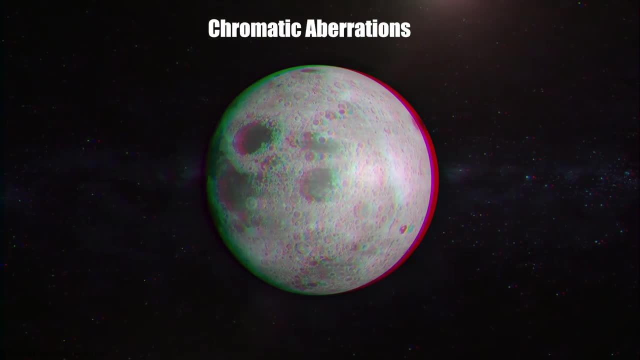 This classification of refractor telescopes is done on the basis of how many wavelengths of light it focuses. Light has three main fundamental colors: red, blue and green. A normal refractor uses a single lens. But with a single lens the telescope produces lots of chromatic aberrations. 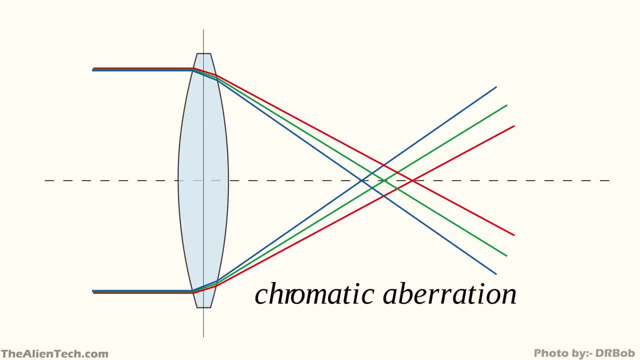 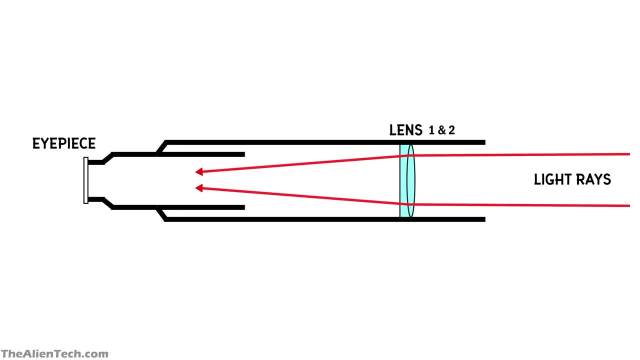 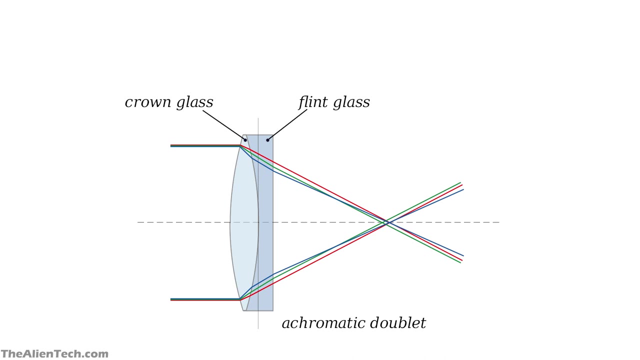 These chromatic aberrations happen because all three colors do not focus on one single point. So to reduce these chromatic aberrations, a second lens is used in these refractors. When these lenses are used, it is called a doublet refractor telescope. 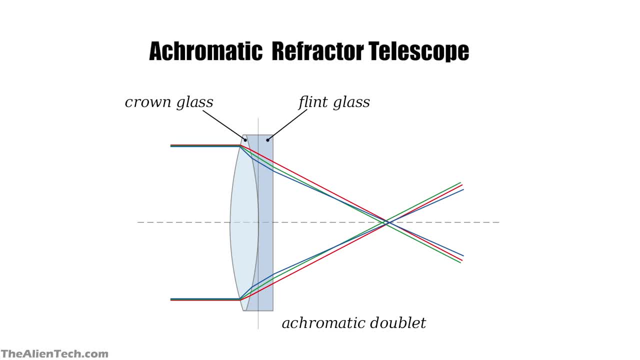 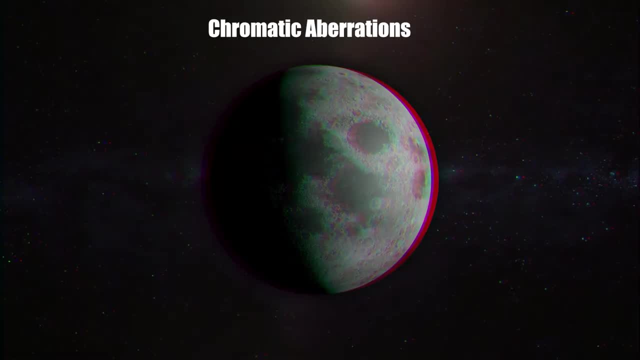 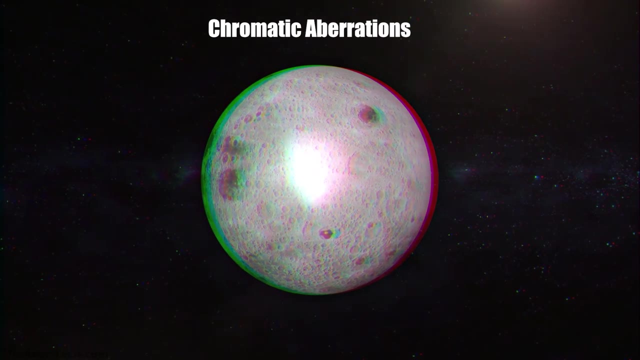 An achromatic refractor telescope focuses two wavelengths of light at a single point. This results in fewer chromatic aberrations. But even with the achromatic refractor there are still some chromatic aberrations you might notice. So to get rid of even those chromatic aberrations, the refractor telescope needs to focus all. 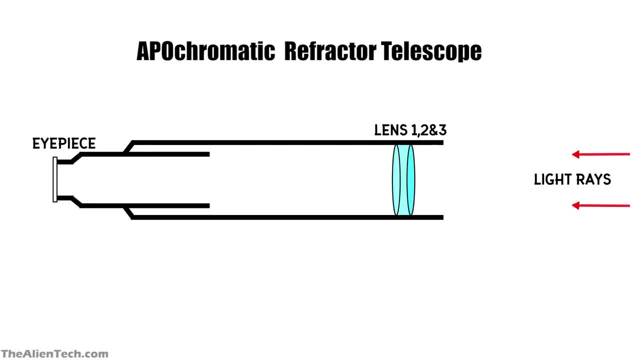 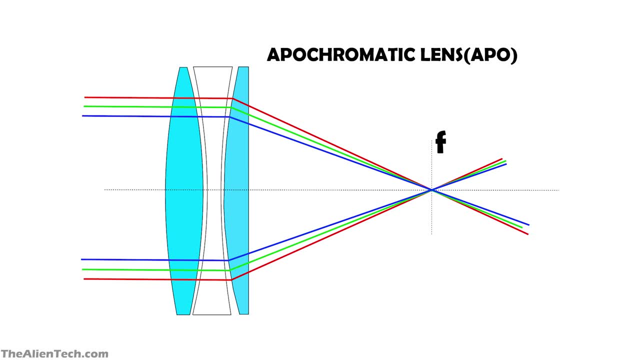 three wavelengths at one single point. The apochromatic refractor telescope does the exact same thing. These telescopes usually use three lenses to focus all three wavelengths at a single point. With advancements in lens technology, it is also possible to achieve this by using only. 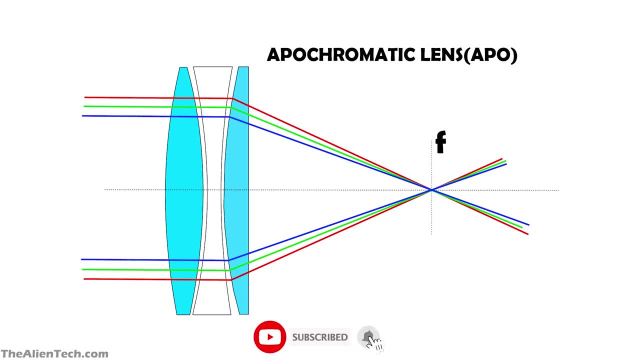 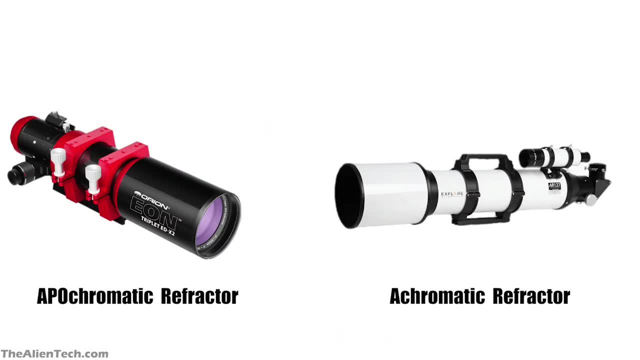 two lenses, But the majority of apochromatic refractors you will find use three lenses. So to get rid of even those chromatic aberrations, the refractor telescope needs to focus all three wavelengths at one point. The apochromatic refractor telescope is more expensive than the achromatic refractor telescope. 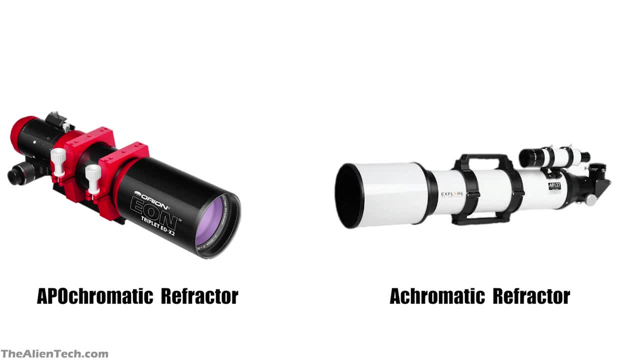 If you just want to observe celestial objects, then your best option is to stick with an achromatic refractor telescope. Apochromatic telescopes usually give better and sharper images, which are good for astrophotography. Most astrophotographers prefer an apochromatic telescope over an achromatic telescope. 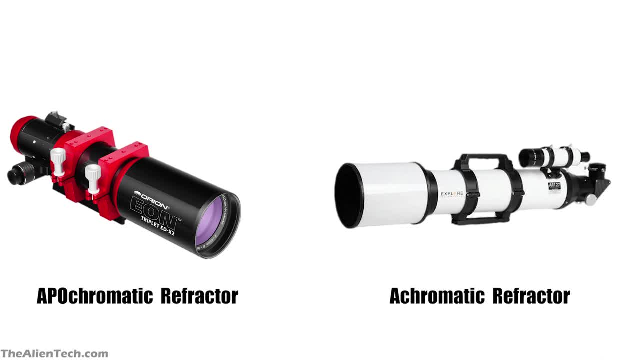 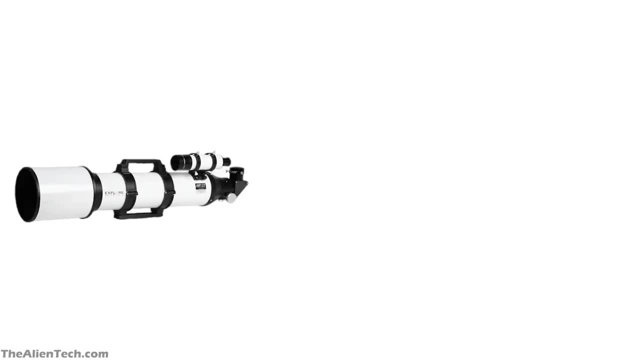 So if you want to do astrophotography, then an apochromatic telescope is for you. Advantages of Refractor Telescopes: The image quality you get with a refractor telescope is good. These telescopes do not need any collimation. 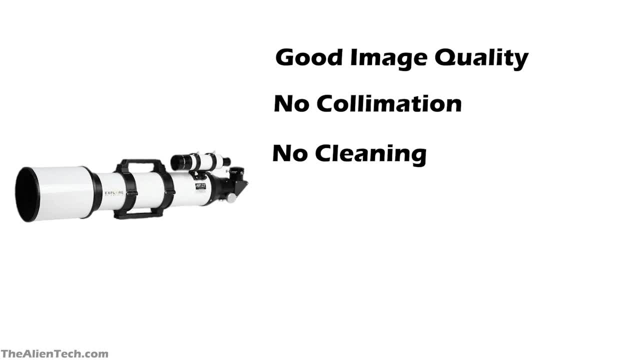 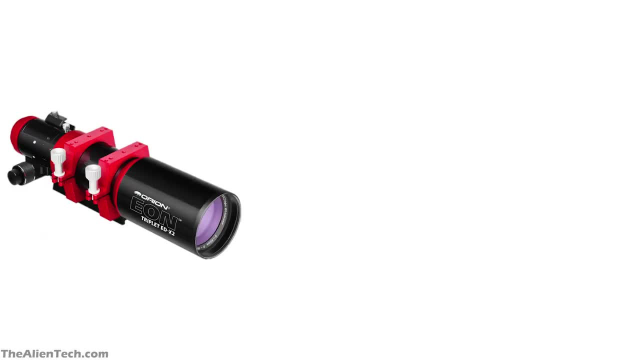 These telescopes are closed-tube telescopes, so they do not need frequent cleaning. Disadvantages of Refractor Telescopes: These telescopes use lenses that cause refraction of light And because of this they suffer from chromatic aberrations. 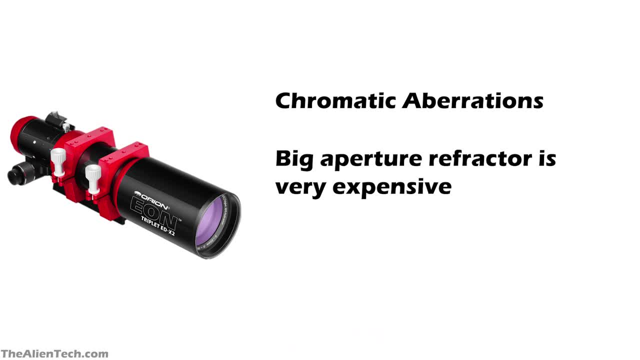 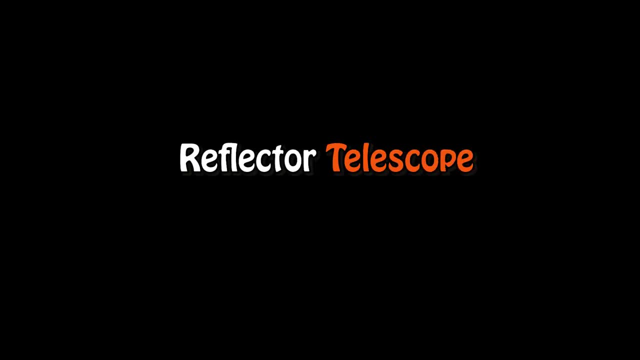 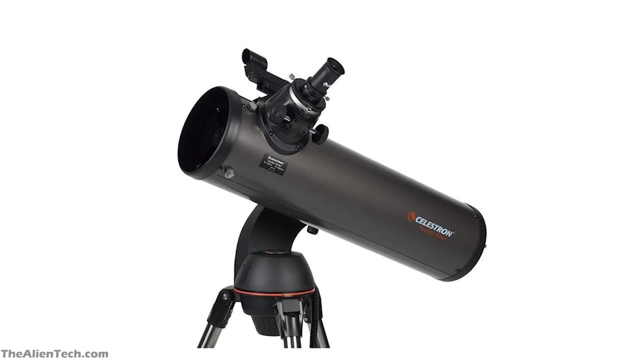 A larger lens is very costly to manufacture, so these telescopes get very expensive with an increase in aperture size. Reflector Telescope- A reflector telescope- does not look like a traditional telescope. These telescopes use mirrors instead of lenses to collect light. The eyepiece of the reflector telescope is at the front. 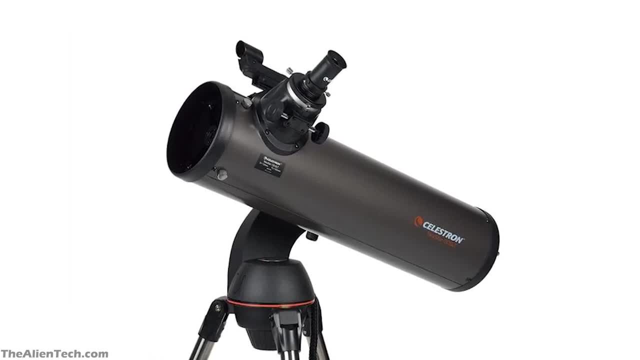 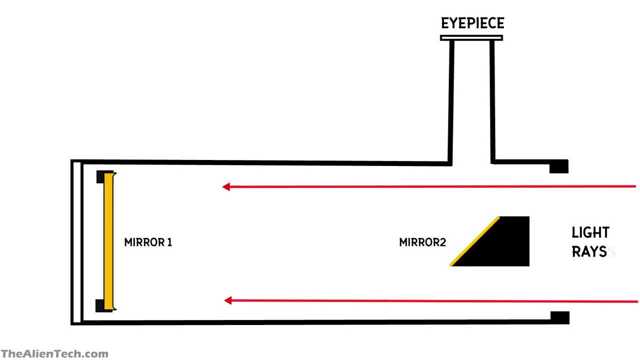 You can recognize a reflector telescope just by the position of its eyes. A typical reflector telescope has two mirrors. One mirror is at the bottom of the telescope. This mirror collects light and then reflects it onto the secondary mirror. From the secondary mirror the light is directed towards the eyepiece or a camera. 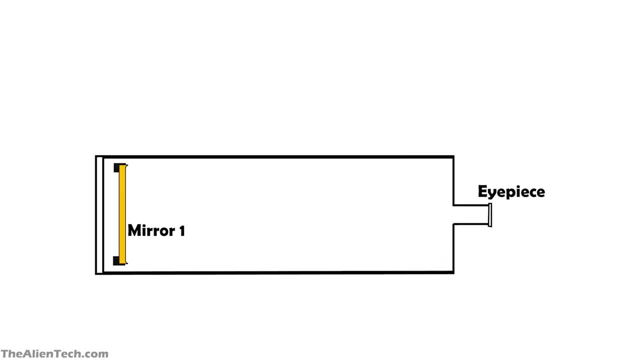 Reflectors are also called Newtonian reflectors. Initially, when the concept of a reflector telescope surfaced, they were thinking of using only one primary mirror and an eyepiece at the front. But this design limits the scope of the telescope. It limited the amount of light collected by the primary mirror, because the person's head